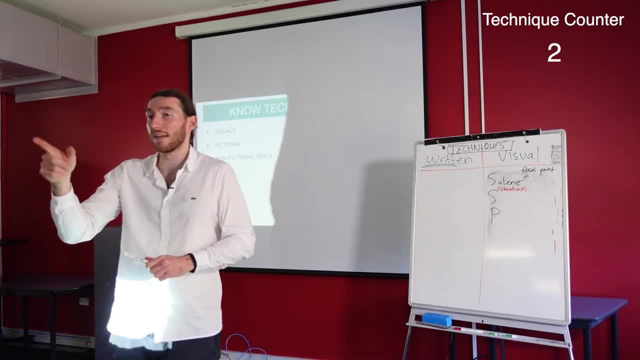 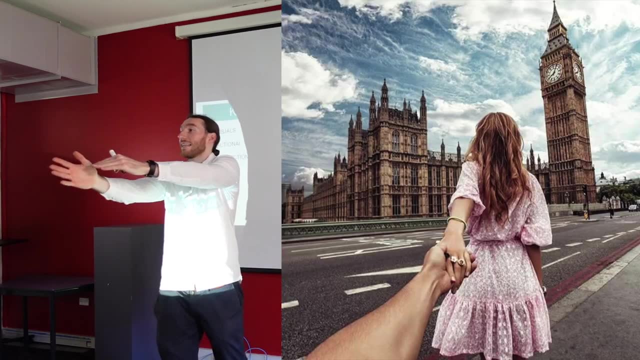 Now, what could make something stand out? Vector lines- great. Vector lines are the lines in an image. take you in to the main part of the image. The vector line could be an arm like extending out in an image. If you see a photo and the camera actually shows the arm going out like that. 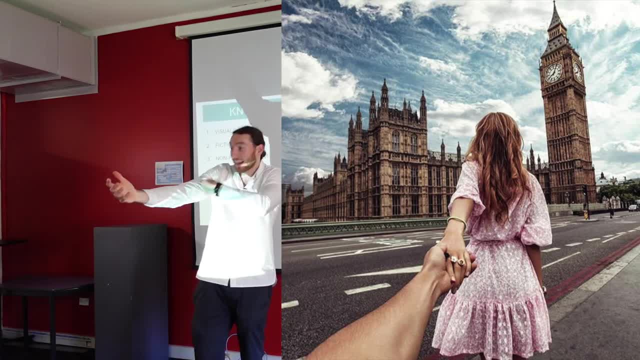 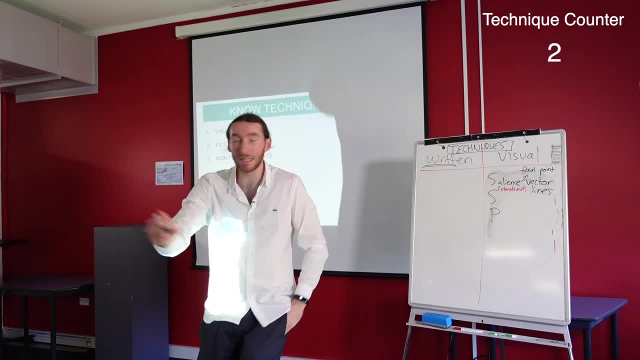 then that is the vector line, taking you to what is salient. but the vector line, the arm. the arm is a vector line. When you speak about salience, you have to say what makes it salient. It might be the vector line. 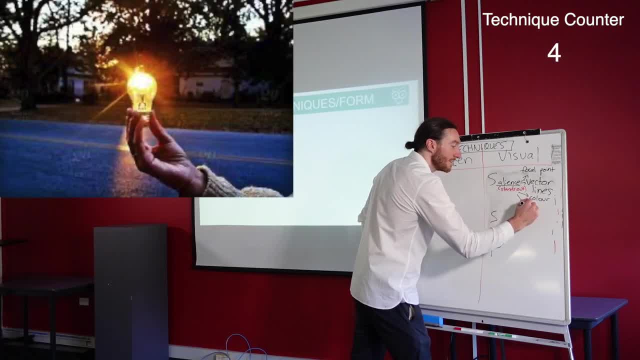 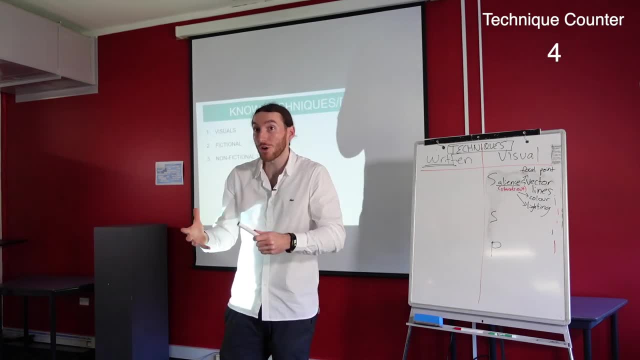 Vector line. what else could you say Colour? we could talk about lighting, but often with these things, it's not just colour or lighting itself that makes something salient. it's what about those things? It's contrast that makes it stand out. So contrasting colours or what is. 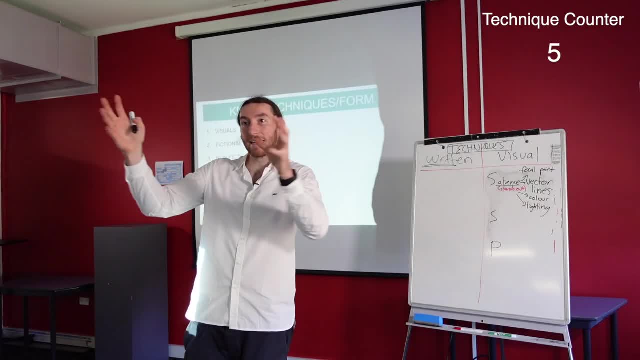 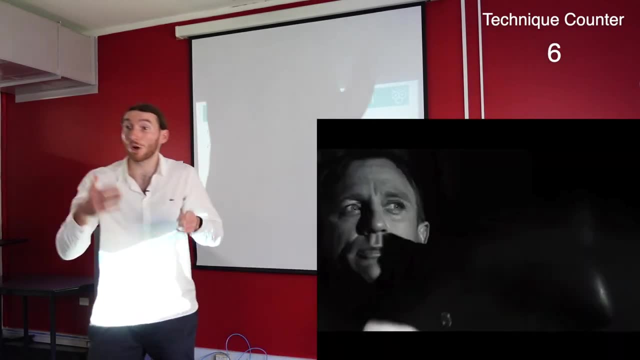 it called when there is light and dark in an image. There's light and dark and the thing that's in the light becomes salient because everything else is dark around it. What's that called? Chiaroscuro? so that is a contrast between light and dark. Very, very common technique: Body language. 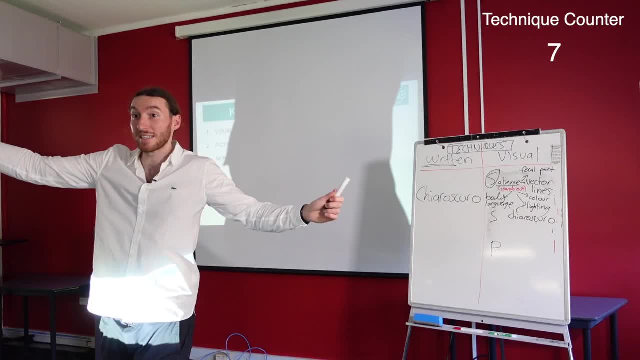 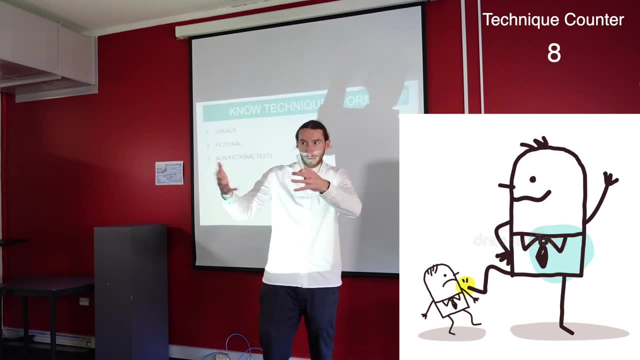 could potentially make something salient If someone was like really expressive, expressive body language. maybe that's making them pop out Size and scale. that goes to the composition right, How it's composed, how it's put together. Often you see something at the front of the image and the 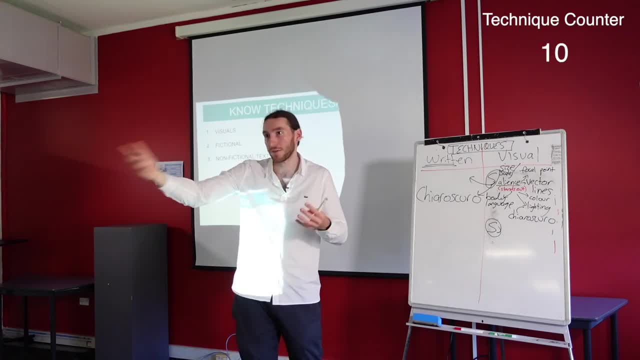 back. what do we call those two things? Foreground, background. So one of those things makes it salient great. Now tell me the effect of it or the significance of it, using a key term from the question. The second S is symbolism. Obviously there might be a kind of symbol in the image. 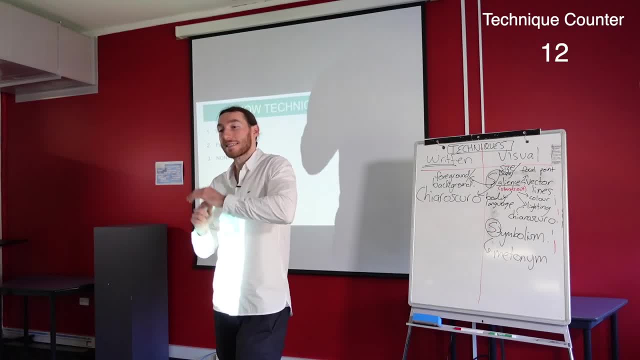 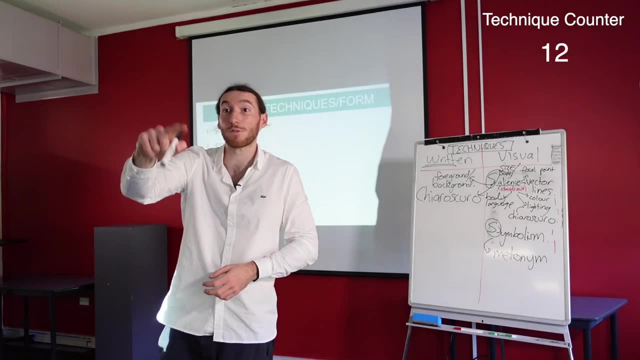 Don't forget about those. A metonym, So that means something represents a larger thing. So a phone is metonymic for technology. So you might want to put in brackets phone arrow technology. Symbolism is more like a thing that is widely accepted. Does anyone know what a dove is? 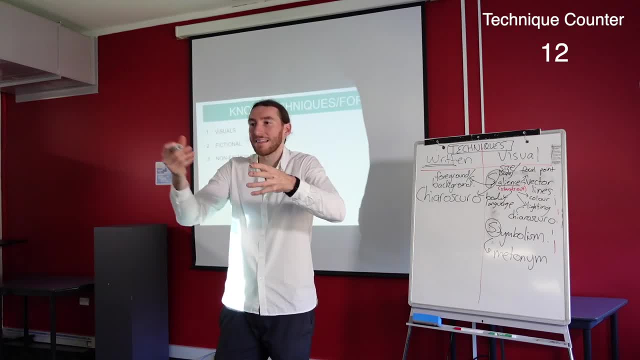 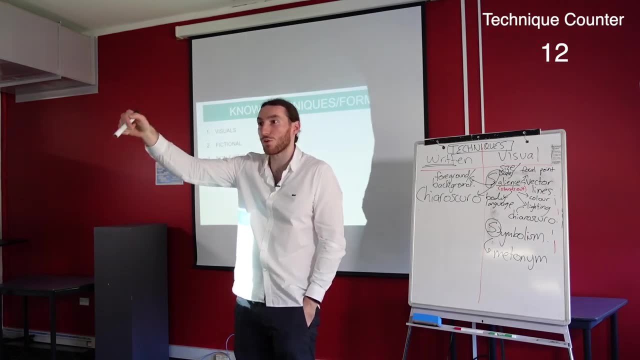 symbolic for Peace. A dove is an object and it links to this concept, Whereas a dove might be metonymic for animals or birds or something. There's a more direct connection between the category. So when something has a category, it's an object. So it's an object, it's an object, So.